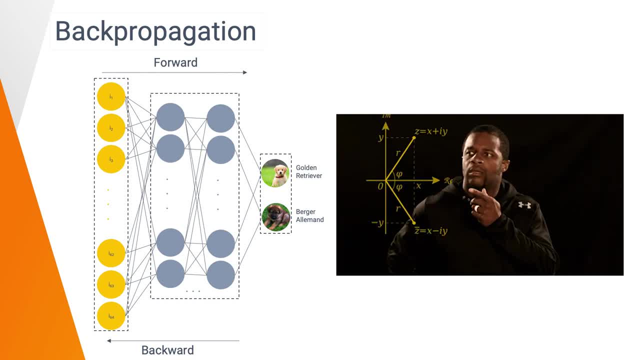 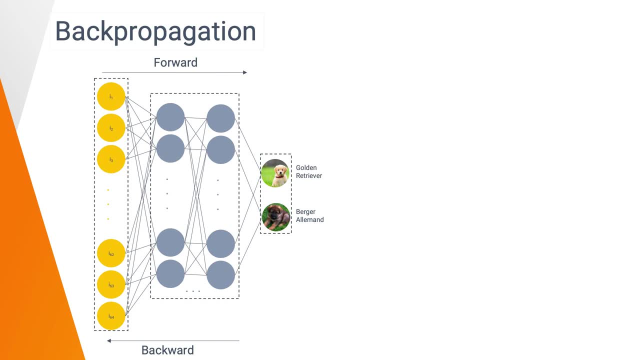 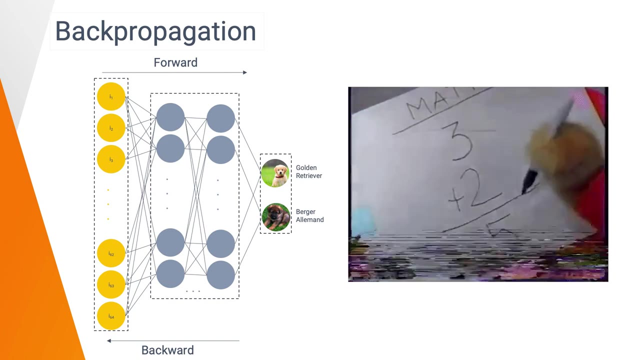 It's an exercise I really recommend to each artificial intelligence engineer. knowing the mathematics hidden behind lines of codes is really important For our demonstration in this video. you just need to know how addition, multiplication and subtraction works, plus partial derivative. Our demonstration will be based on a simple neural 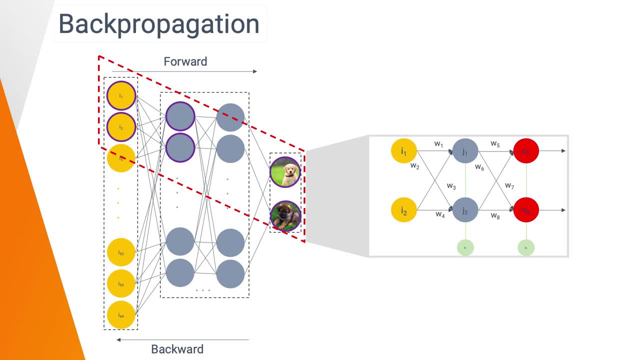 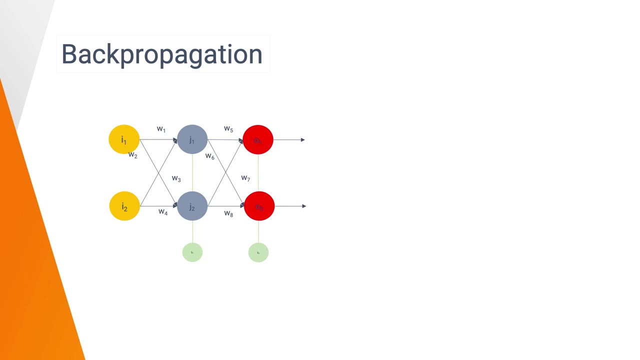 network. My inspiration for this demonstration has come from Matt Mazur. Do not hesitate to check his blog post in the description of this video. So the neural network we will use as one input layer, one hidden layer and one output layer, with two neurons on each. We will feed. 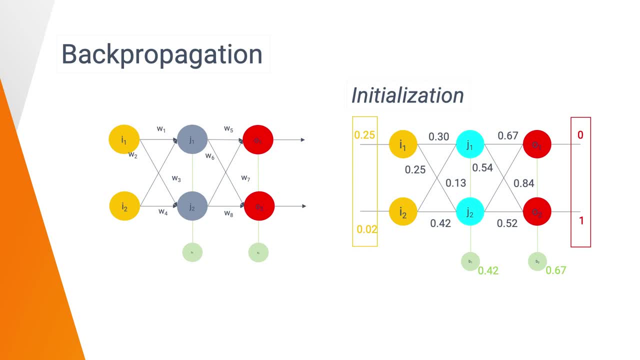 our neural network with two numbers here in yellow, and we are looking to predict 0 and 1 here in red. First of all, we initialize the weights of our neural networks randomly. We also set a bias in each layer here in green. The first phase here is the forward propagation. 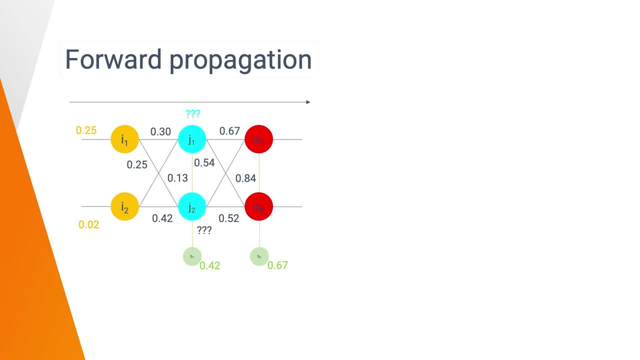 We will, in this phase, find the value for each neuron. here in blue. We will calculate the value of the G1 neuron. In order to do so, we will use the two inputs and the two edges connected to G1.. We calculate the value of G1 by this formula. A really simple formula, isn't it? 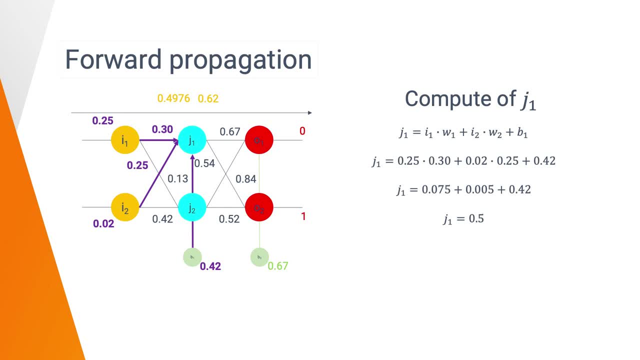 We replace all the values and we obtain 0.5 for G1.. But the work doesn't end here. 0.5 is the value for G1 in the network, But now we need to calculate the value G1 will deliver to the rest of the network. 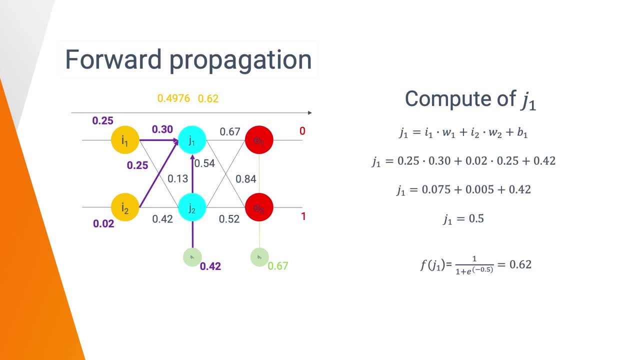 To do so. most of you know that we are going to use what we call the activation function in order to break the linearity of our neural network. We will use here the sigmoid function as our function activation and we obtain as output for the neuron G1,. 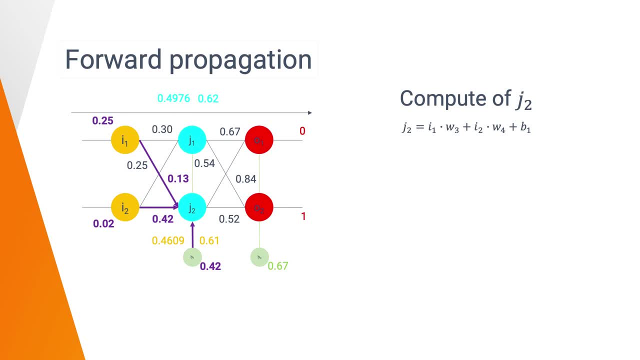 0.62.. We repeat exactly the same process for G2. But please note that we change the edges and by doing so the values. Here we use W3 and W4 as weights. Here the output of G2 is 0.61, and the input around 0.46. 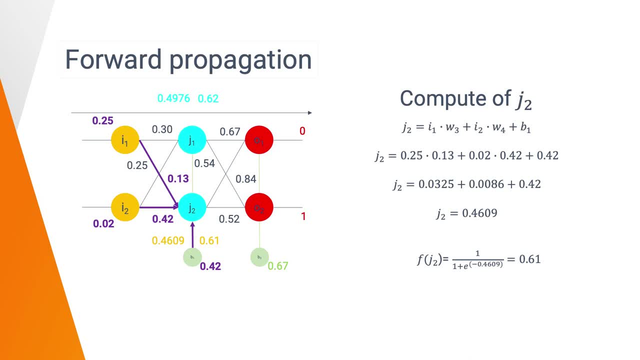 We can update our schema with those new values. Now we can calculate the values of our output layer. That is our output layer That we will compare later to our targets. We hope here to get as close as we can to 0 and 1.. 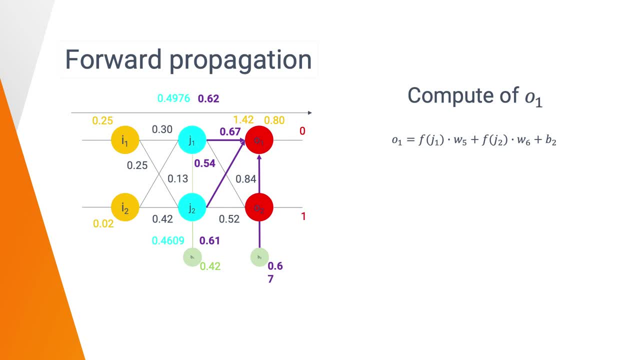 But as the initialization was random, we will have to be very lucky. The formula is, exactly like previously, The symbol combinatorial formula of the sum of the input multiplied by their respective weights. Exactly as previously, here we can calculate the input and the output of each neurons. 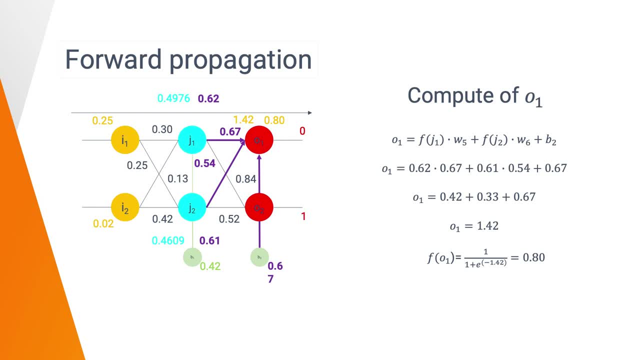 of our output layer. For O1, we got 1.42 as input and 0.80 as output. Following again the same process for O2, we got 1.51 and 0.82.. We can also report all those values on our schema. 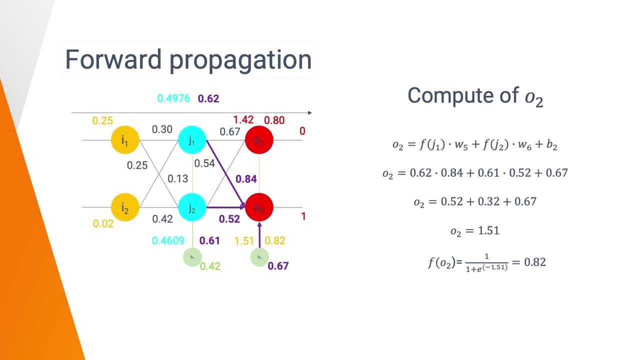 Do not hesitate to pause this part of the video and try to retrieve the same numbers. You can also put new weights values at the initialization and change the value of input and output and feed your own neural network. Now that we have calculated those values, we can notice that we have not been lucky at all. 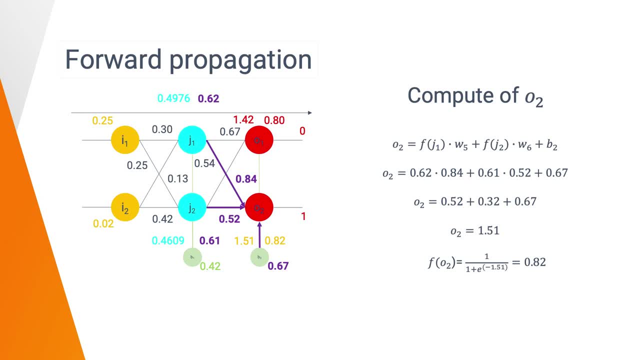 Instead of getting 0, we got 0.80.. And instead of getting 1, we got 0.82.. This second value is not too bad. however, Now the real work of the backpropagation algorithm can start. 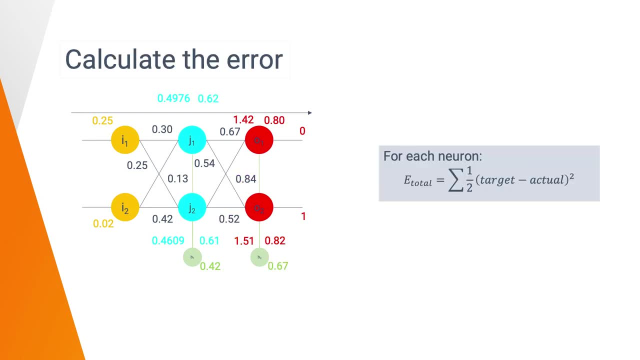 We will calculate the error. We will calculate the error of each part of our neural network and adjust the weights to get closer to the values desired in output. Here in this video, we will just do one iteration, because it could take hundreds of iterations before getting to the value we want. 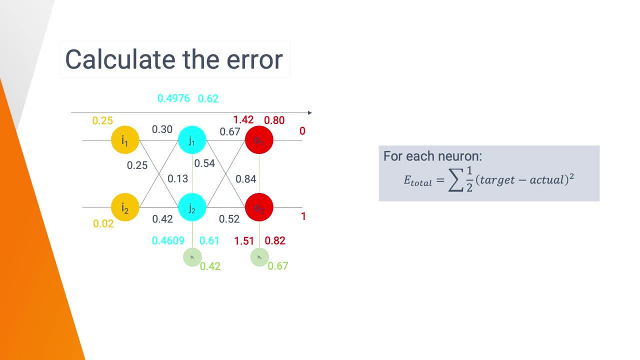 But do not worry, In the next video we will implement this method in TensorFlow and we will see how machines are our friend. to be quicker Here, we will calculate the error for each neuron. We can decide to remove the half if we want here. 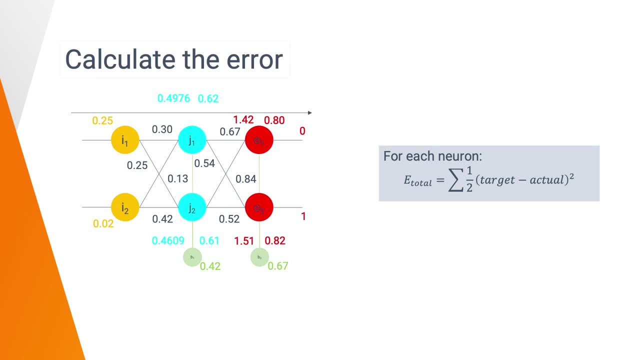 Here we introduce half to cancel the times 2 introduced later by the derivative of the error. So it is just for simplification and it doesn't matter if we introduce a constant here, as the error will be multiplied anyway by the learning rate that we will see later. 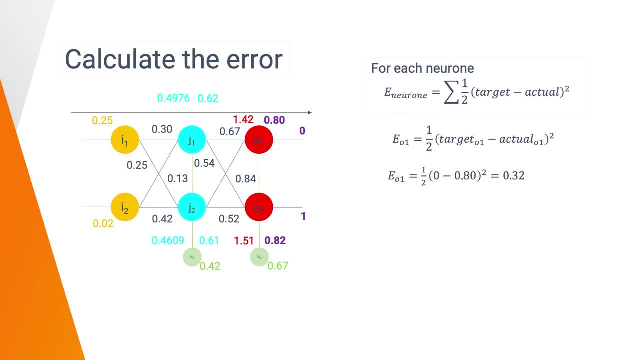 So we calculate the error For the output layer. here, the value we were expected was 0 and we got 0.80.. So the error of 01 is 0.32. using this formula, Doing the same for the error of 02, we got 0.0162.. 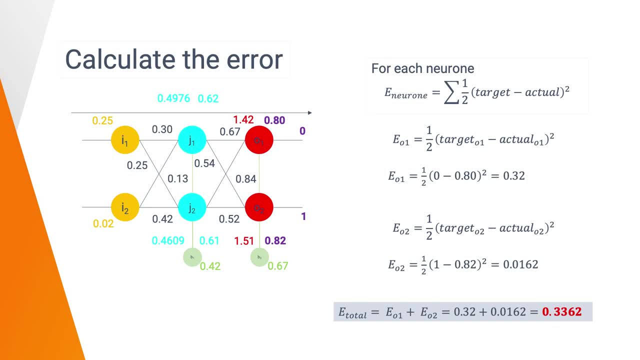 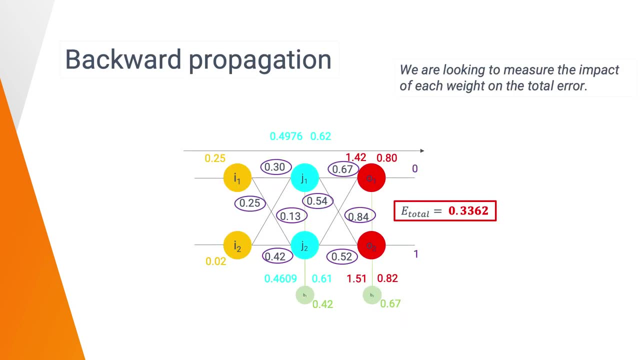 So the total error of this first iteration is 0.4362.. Now that we know this total error, we are going to try to find the impact of each weight in order to reduce this error in the next iteration. So we will calculate the impact of weight 8 here on the total error. 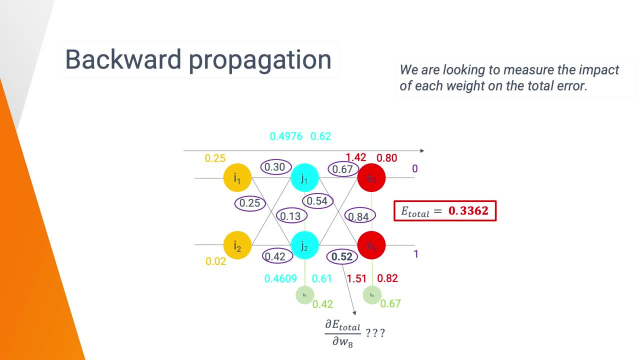 It is what we call the partial derivative of E total on W8. We can also call it the gradient with respect to W8. And later we can calculate the same for W4, and for any other weight of any other layer in our network. 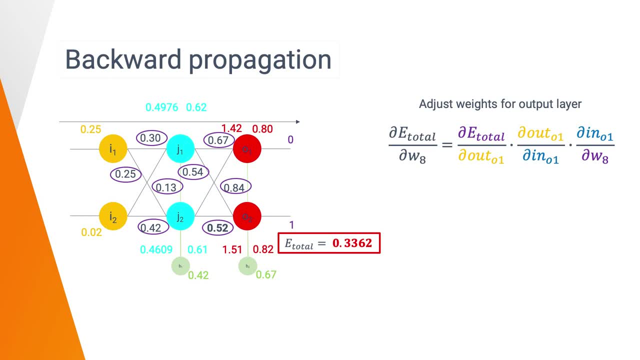 So let's calculate the impact of W8 on the total error by applying the chain rule. You can refer to the Wikipedia article if you need it, or you can trust me: We can write this formula Visually. it is what we do. 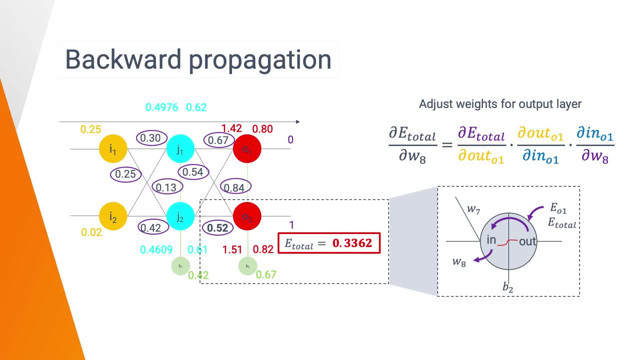 To calculate the impact of W8 on E total, we need to go back through each step of compute that allowed us to calculate the error total during the forward propagation. For the first part, we had previously defined the error of O1 and O2,. 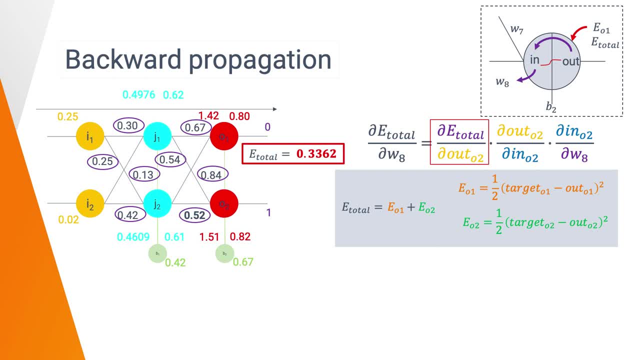 and we defined the total error as the sum of the O1 error and the O2 error. So we can derivate this formula with respect to the output of O2.. And we got only terms where O appear. Do not hesitate to pause the video and to calculate on your own this derivate function. 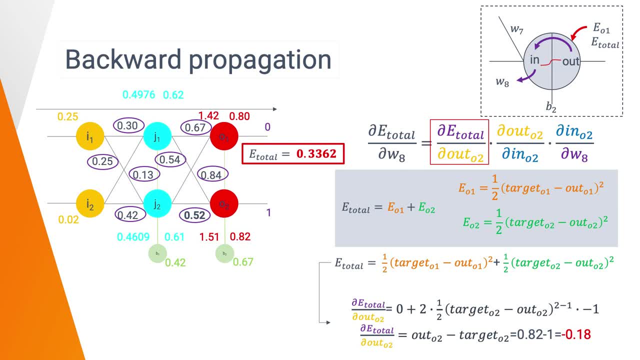 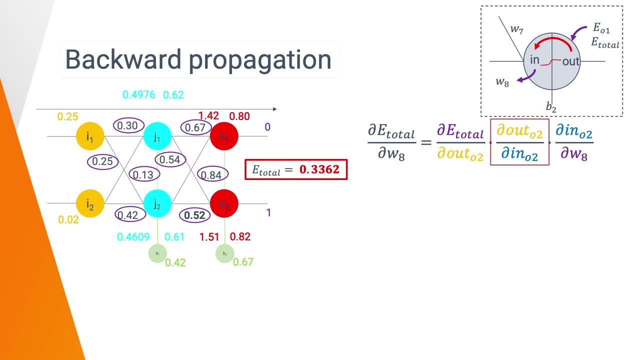 Here we got as value minus 0.8. Let's get on the next term, which is really simple to compute, as between the input and the output of our neuron, we only have the activation function Here, the sigmoid, as remainder. 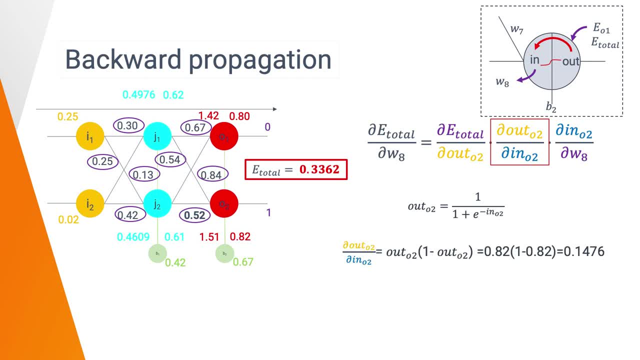 So we just need to derivate the sigmoid function And we obtain this really simple formula which lead us to a value of 0.1476.. And finally, we need to retrieve the impact of W8 on the input of O2.. 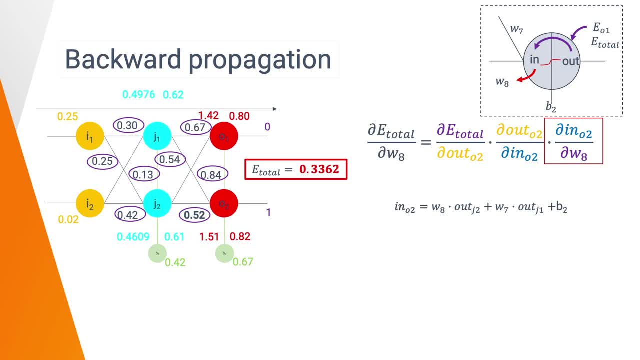 To do so, we took the formula of the input of O2 that we previously used, and we derivate the formula with respect of W8. And we only got the output of the neuron G2, which is 0.71.. So by combining all those terms, 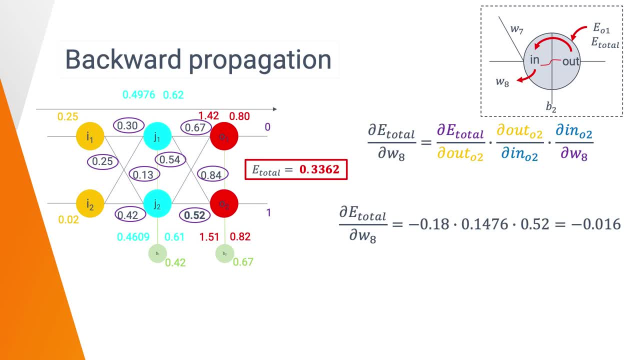 we can retrieve that the partial derivative of E total with respect of W8 is minus 0.016.. Now we can calculate the updated value of W8, which is the value of W8 minus the learning rate, which multiplies the partial derivative we just calculated. 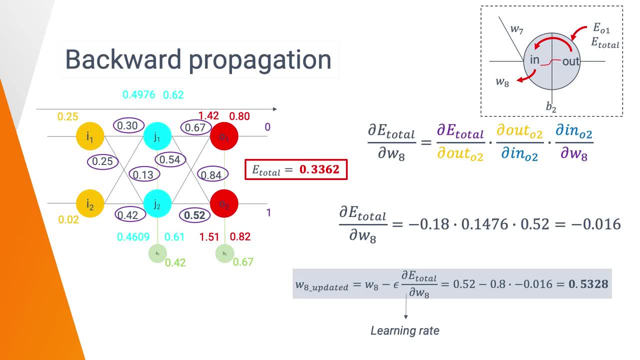 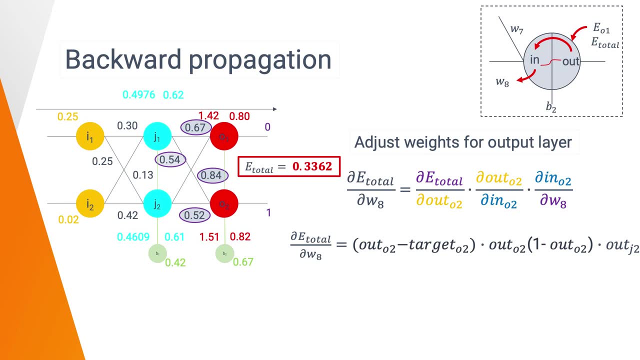 And we obtain a new value of 0.3328 to compare to the previous one of 0.52.. Through this compute, we can simplify the formula to calculate the partial derivative for each weight. We can now compute the updated value for each of the weights on this layer. 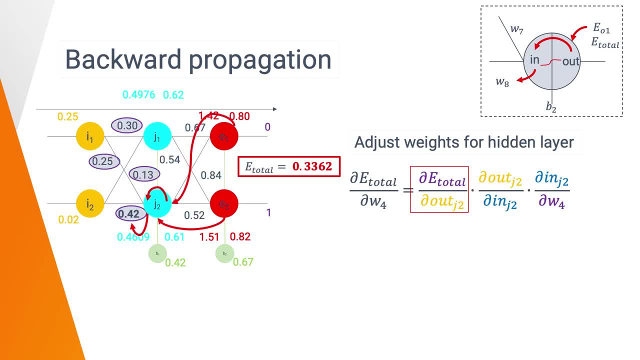 I recommend you to do that by yourself. Now that we have seen how we can apply the back propagation on an output layer, let's apply the algorithm to an hidden layer. Here we are going to compute the new value for W4.. So, as previously, with the chain rule, 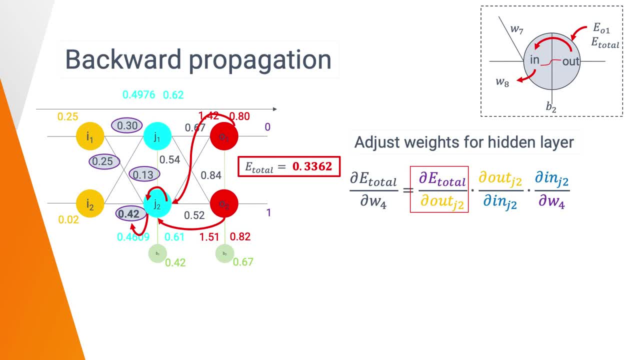 we can write the partial derivative of the error total with respect of W4 as this formula: First we can decompose the partial derivative of error total as the sum of the partial derivative of the error O1 and O2.. And then we can decompose each partial derivative. 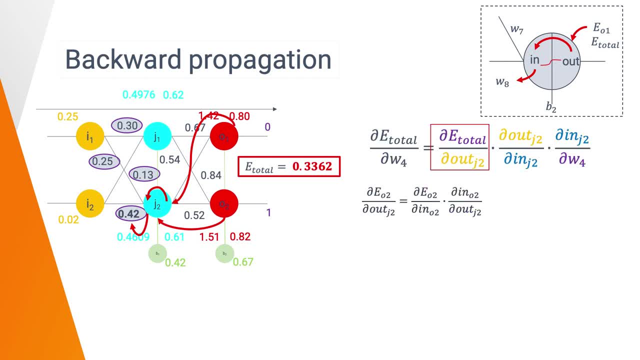 We can notice that more we go back deeper, more the complexity increases. Imagine doing so for a layer of hundreds of neurons in a network of thousands of layers. It is why we have deep learning frameworks such as TensorFlow that we will use in the next video.